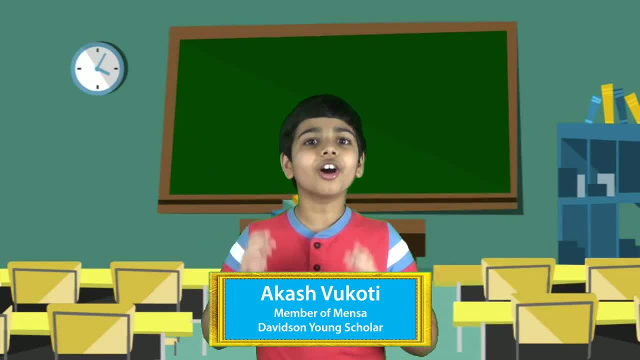 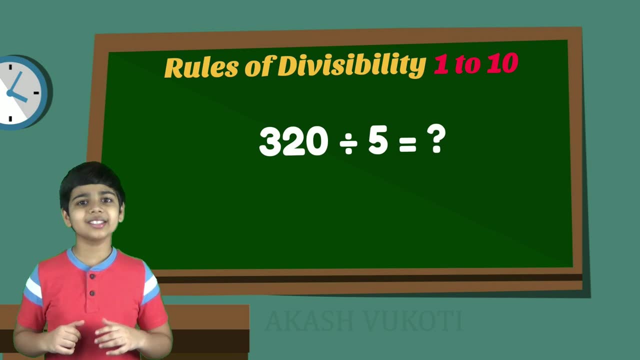 Hello friends, I'm Akash and a hearty welcome to my YouTube channel. If you want to know whether 320 is divisible by 5, then you don't actually have to physically divide 320 by 5.. In fact, you can just use something called the rule of divisibility by 5 and you can figure it out. In this case, the rule of divisibility by 5 is that if the number ends in either 0 or 5,, then the number is divisible by 5.. 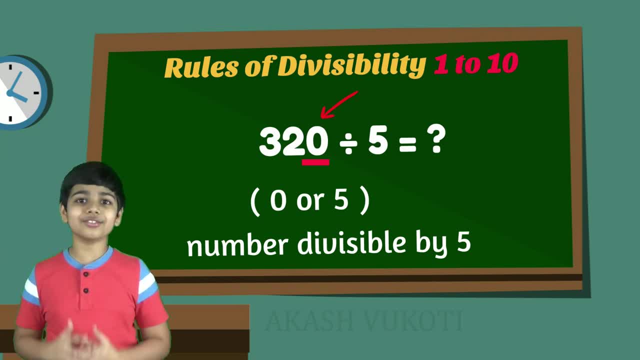 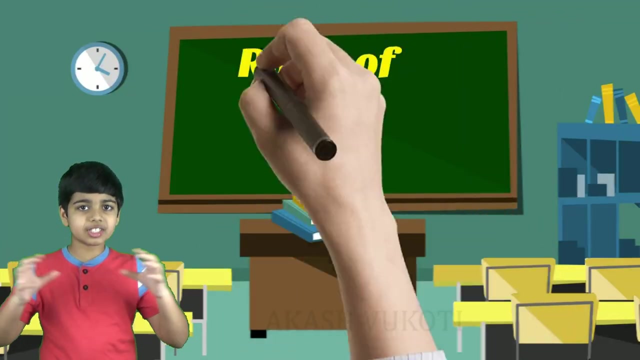 Now, 320 is divisible by 5, because it ends in 0.. Now these rules will be very, very helpful in figuring out if a number is divisible by any number, from 1 through 10.. So in this video, we are going to learn the rules of divisibility from 1 to 10.. 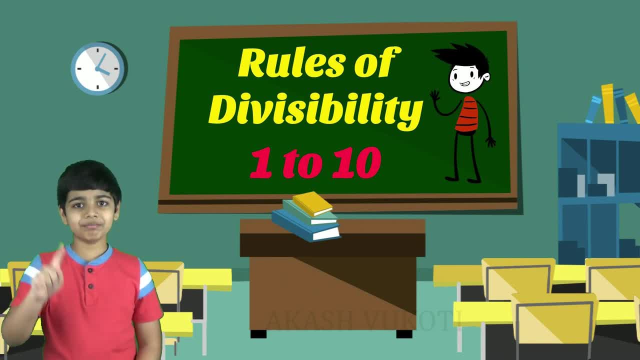 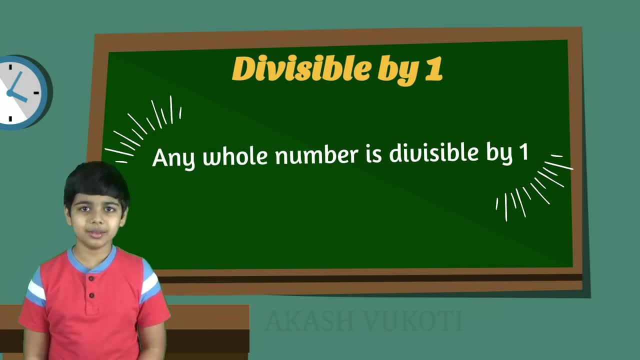 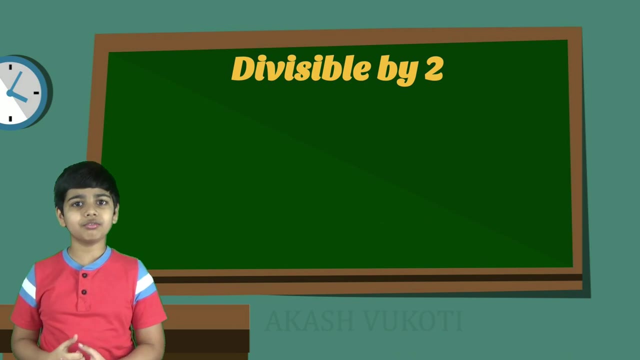 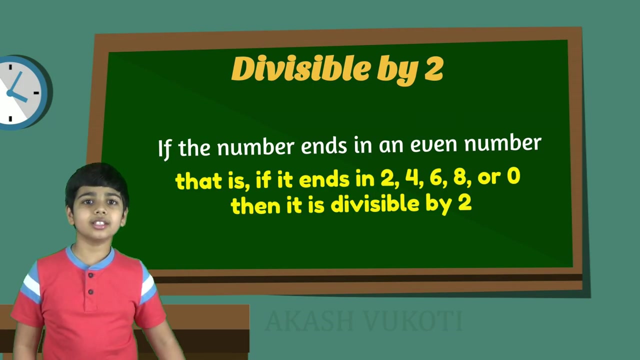 Now let's begin with 1.. This is obviously the most simplest one of them all, Because any whole number is divisible by 1.. So let's move on to the number 2.. The rule of divisibility for the number 2 is if the number ends in an even number, that is, if it ends in 2,, 4,, 6,, 8, or 0,, then it is divisible by 2.. 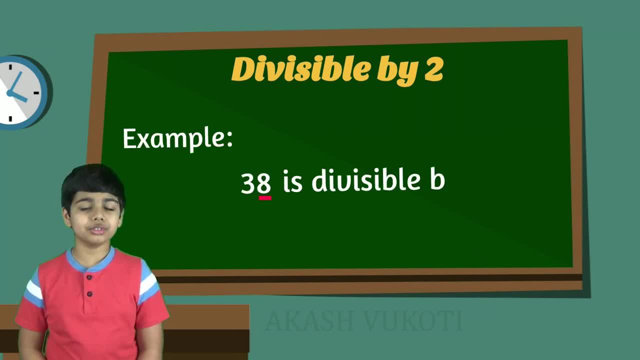 For example, 38 is divisible by 2 because it ends in 2.. For example, 38 is divisible by 2 because it ends in 2.. For example, 38 is divisible by 2 because it ends in 2.. 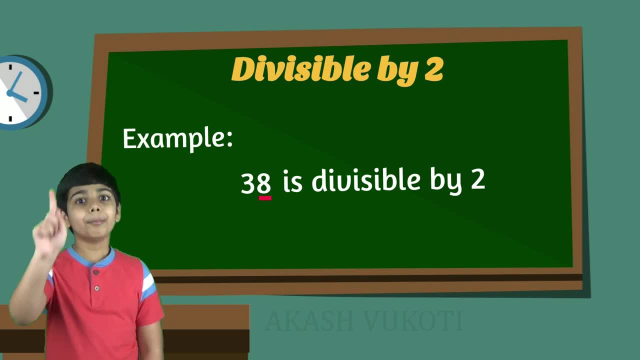 For example, 38 is divisible by 2 because it ends in 8,, and that's one of the numbers here. For example, 38 is divisible by 2 because it ends in 8,, and that's one of the numbers here. 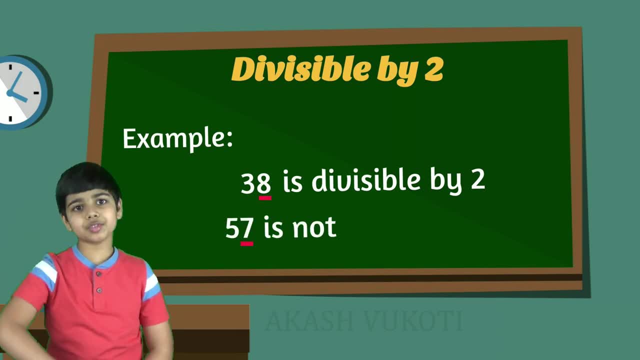 But 57 is not divisible by 2 because it doesn't end in 2,, 4,, 6,, 8, or 0. It ends in 7, so it's not divisible by 2.. For 3, you add up the digits of the number. 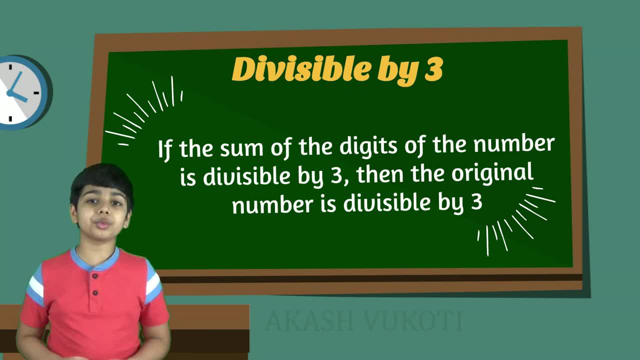 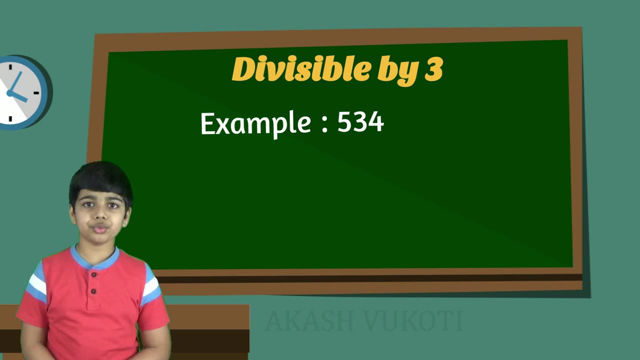 and if the resulting number is 2, is divisible by 2.. is divisible by 3, then the whole original number is also divisible by 3. for example, let's try to check: if 534 is divisible by 3, 5 plus 3 plus 4 is 12 and 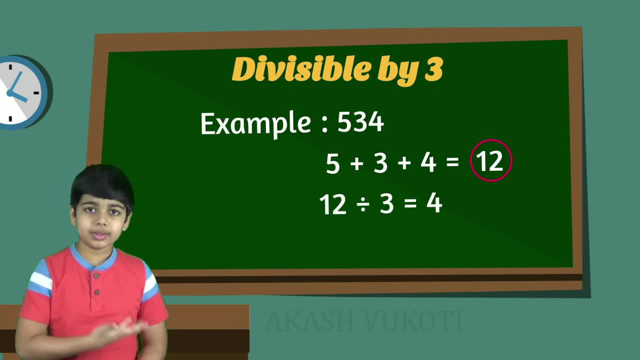 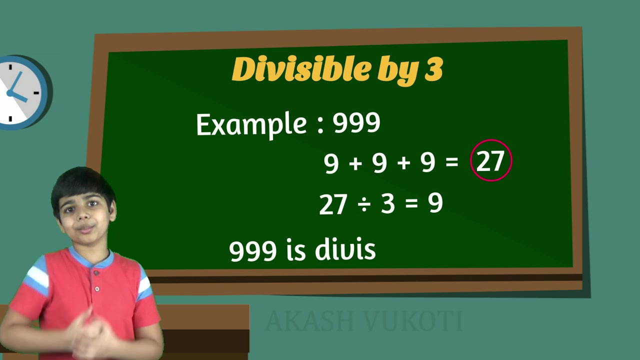 we know 12 is divisible by 3. it's 3 times 4, so 534 is divisible by 3. we wanted to try 999. then we have 9 plus 9 plus 9, which is 27. we can confirm that 999, the original number, is also divisible by 3. 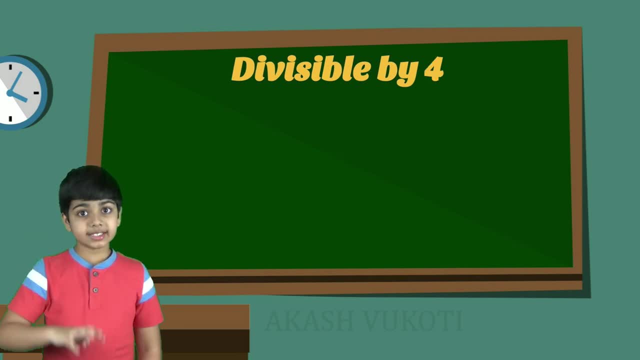 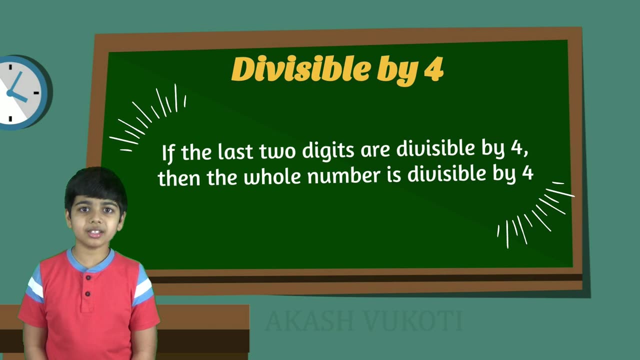 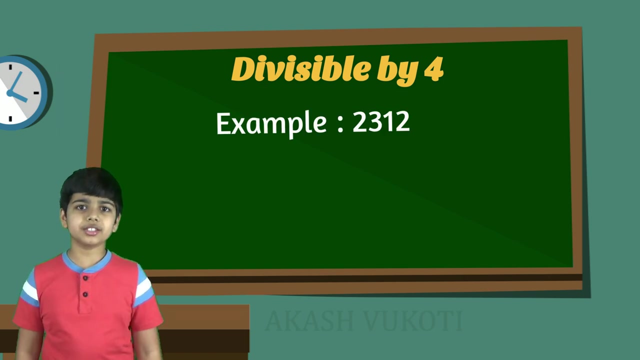 next, for 4. if the last two digits are divisible by 4, then the whole number is divisible by 4. for example, if we wanted to check, say, whether 2312 is divisible by 4, well, we just checked the last two digits, which is 12, 1, 2, and since 12 is, 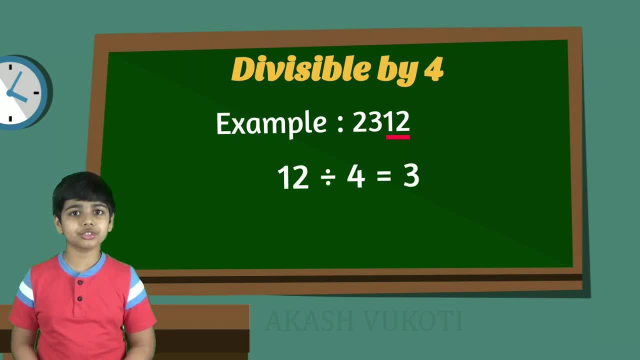 divisible by 4, we can confirm that the original number is 2312 is divisible by 4.. However, for smaller numbers, it's also a useful quick check, which would be to halve the number twice and see if it still remains a whole number. 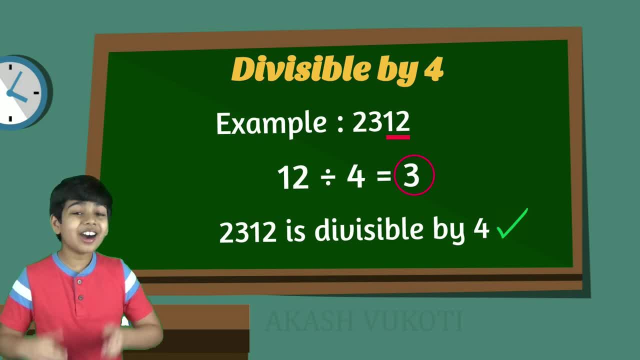 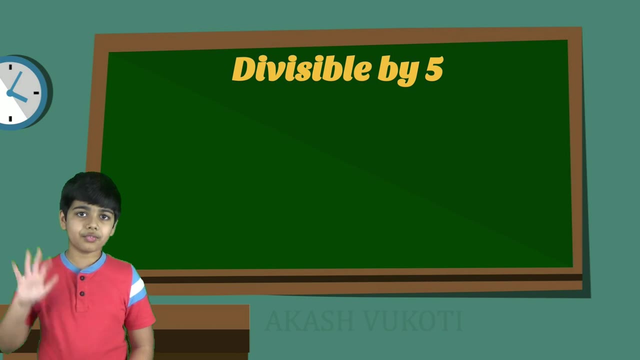 If it is, then it's divisible by 4.. But otherwise, if it has decimals at the end, then it is not divisible by 4.. Now for 5.. Like I explained earlier, the rule of divisibility for 5 is that if the number's last digit is either 0 or 5,. 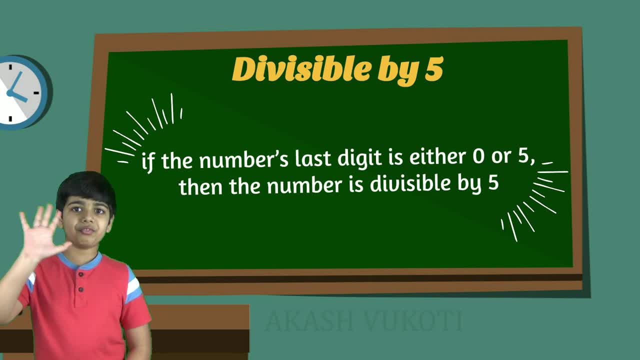 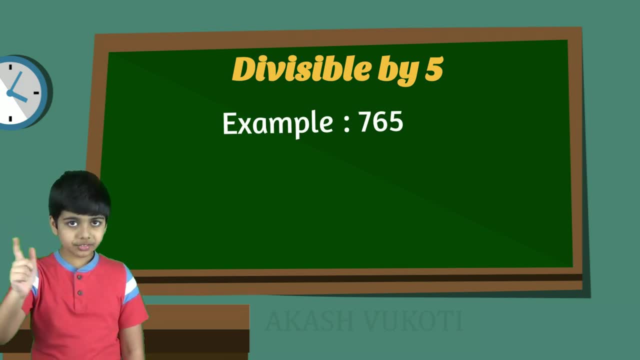 then the number is also divisible by 5.. For example, let's try to check 765.. 765 ends in 5.. So it's divisible by 5.. 154,, though, is not divisible by 5, because it doesn't end in 0 or 5.. 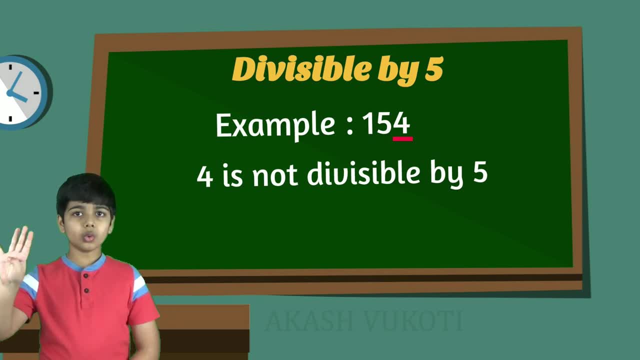 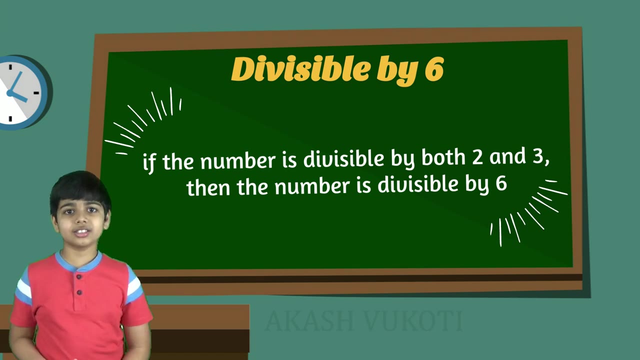 It ends in 4.. So it's not divisible by 5.. 6 is very simple if you know the rules for 2 and 3.. Because 6 is just 2 times 3,, all you have to do is write it down. 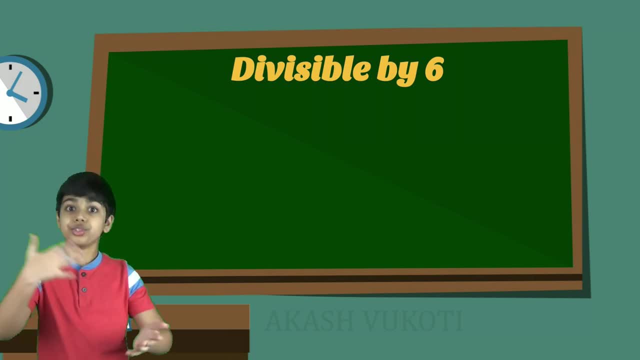 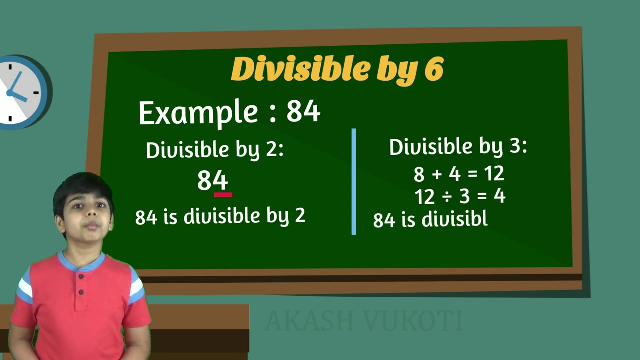 So what you have to make sure is that the number passes both tests. So, for example, 84 is both an even number, so it passes the rule of 2, and its digits add up to 12, which is divisible by 3. So it passes the rule of 3.. 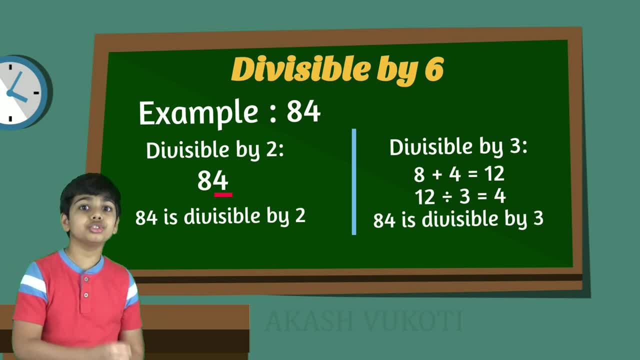 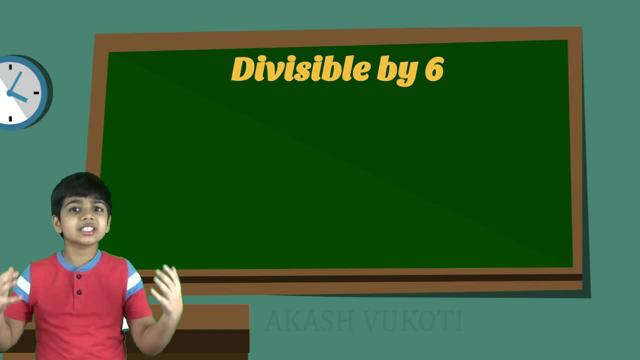 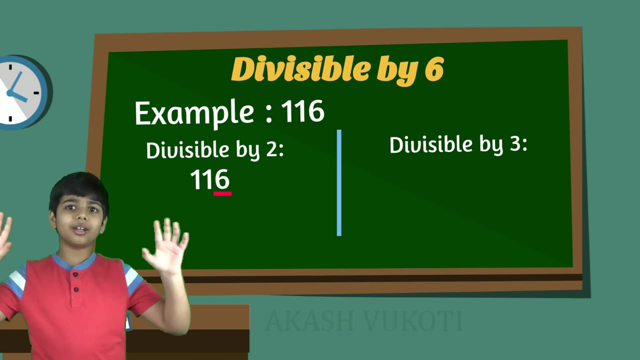 Therefore, if 84 is both divisible by 2 and 3,, then it's divisible by 6.. If it goes 116, then it isn't divisible by 6, because, although it is an even number which passes the rule of 2,. 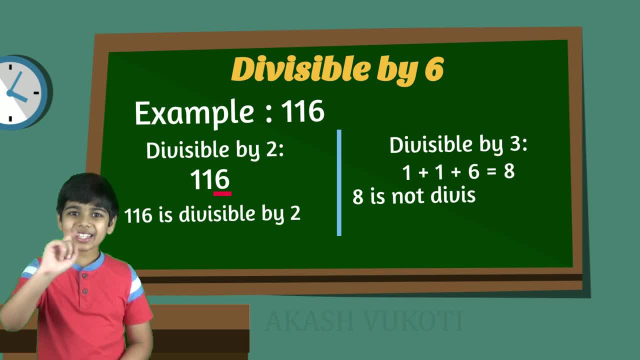 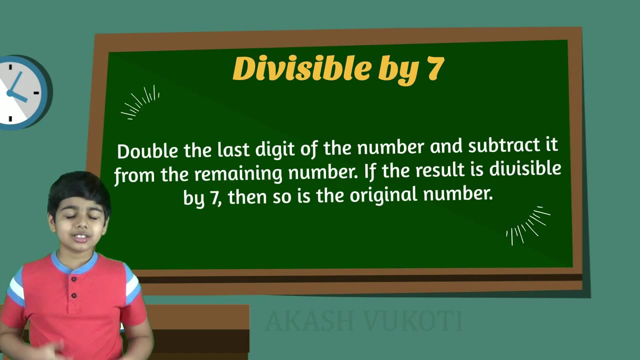 1 plus 1 plus 6 is 8, and 8 is not divisible by 3. So 116 is not divisible by 6.. Now moving on to number 7.. the last digit of the number. then double it and then subtract it from the remaining number. 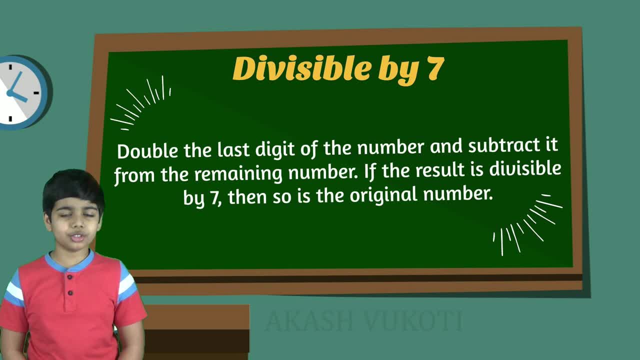 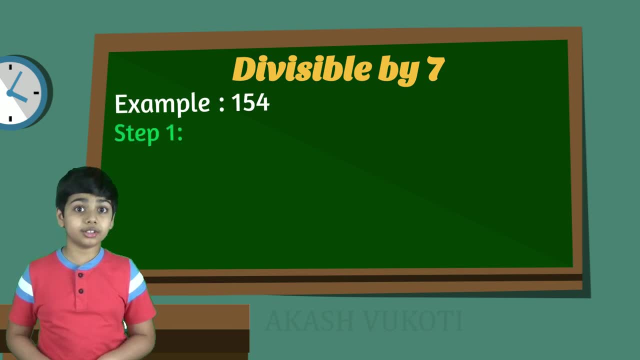 If the result is divisible by 7,, then so is the original number. For example, let's take 154.. The last digit of 154 is 4, and 4 times 2 is 8.. Now, if we subtract 8 from 15,, 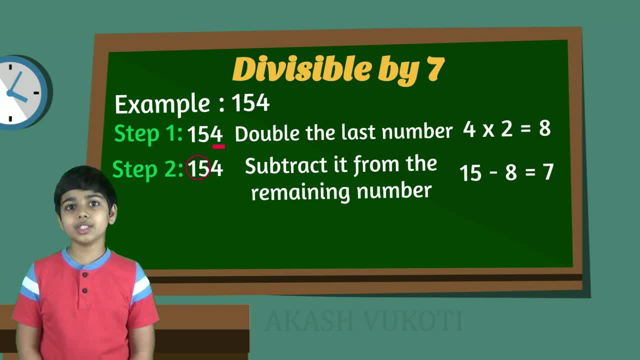 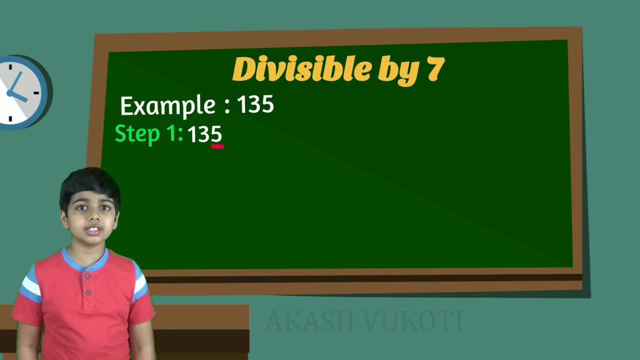 then we get 7, and 7 is divisible by well 7.. So 154 is divisible by 7.. However, let's try taking, say, 135.. The last digit of 135 is 5, and 5 times 2 is 10.. 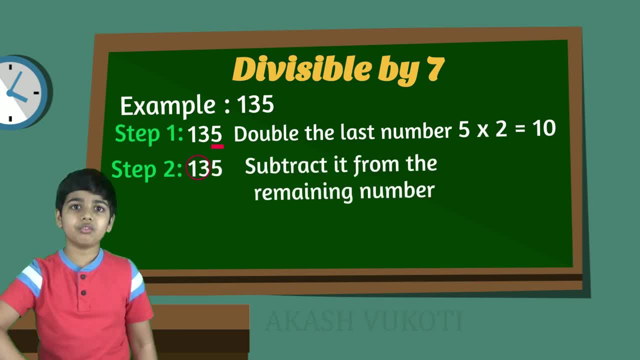 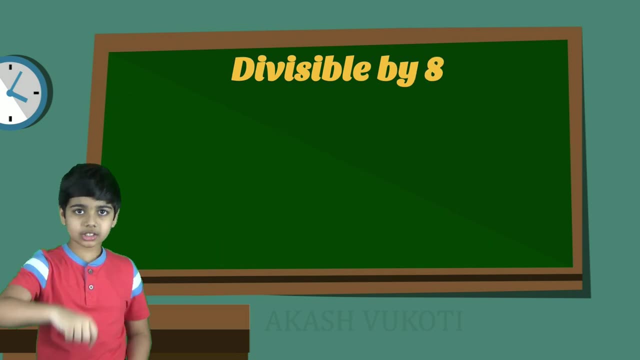 Now, if we subtract 13 from 10,, we get 3,, and 3 is not divisible by 7,, which means that 135 is not divisible by 7.. Coming to 8. 8. It's similar to 4 in that, in this time, if the last three digits of a number 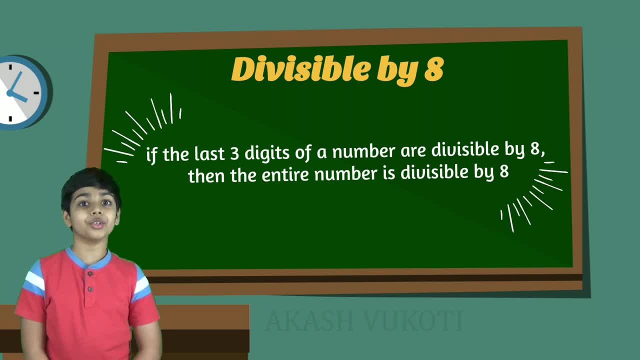 are divisible by 8, then the entire number is divisible by 8.. However, for those last three digit numbers it's kind of hard to understand and check if it's actually divisible by 8.. So there is a quicker method: Just divide by two, 3 times, and if the number is still a whole, 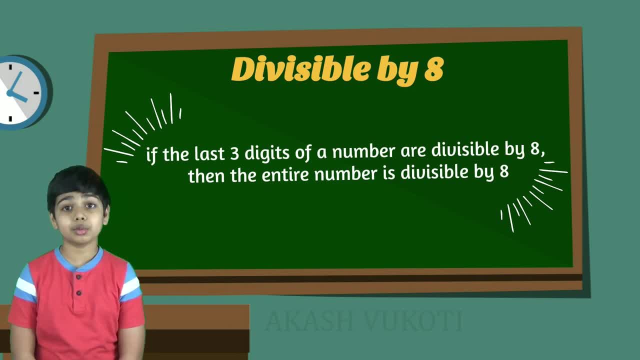 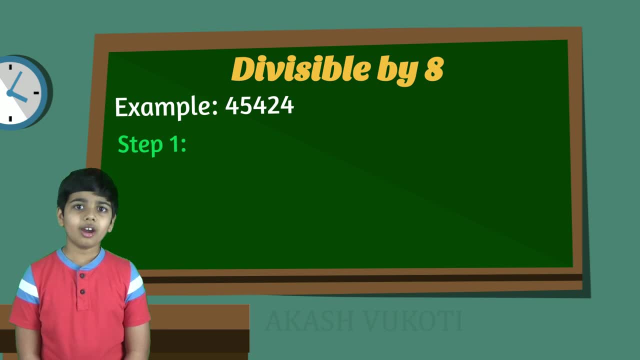 then it's divisible by 8.. For example, the last three digits of 45,424 are 424.. Now, 424 divided by 2 is 212, and 212 divided by 2 is 106.. Curtis, find a number that suscribes you. If the last number 3 in this equation is divisible by 1 over 45,, dividing this number by 2 is 12.. And the last digit of 25,000 already sees a 4, and these are divisible by 8.. Now again, the last 3 are: divisible by 절�icians. For example, 45,424 divided over 12 is 412.. The last number of 244 is 424.. Dividing this number by 2 is 3.. Now, if the last digit is divided by 2 is 424, and the last digit is 12, divided by 2 is 12.. 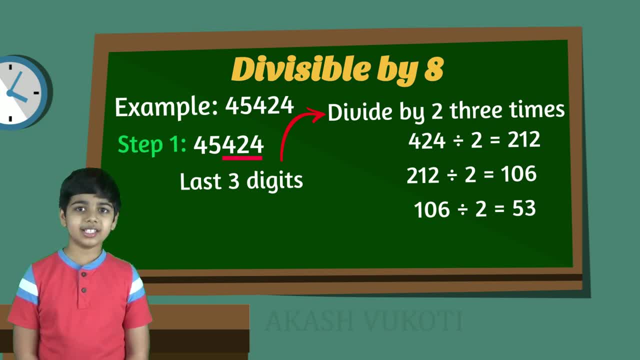 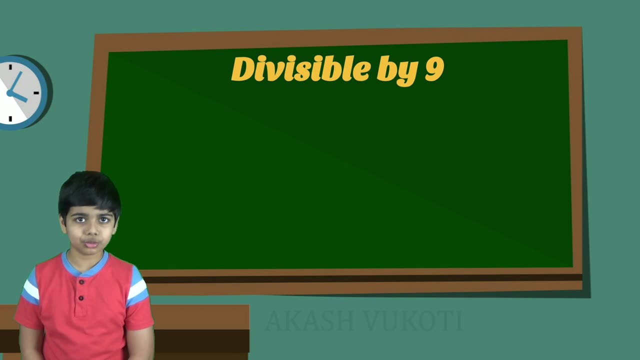 by 2, one last time- results in 53. And 53 is a whole number, which means that 45,424 is divisible by 8. Then to 9.. This one is very similar to the rule of divisibility by 3, in that you add up the. 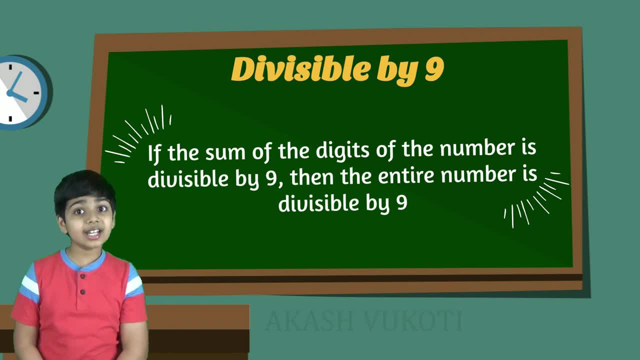 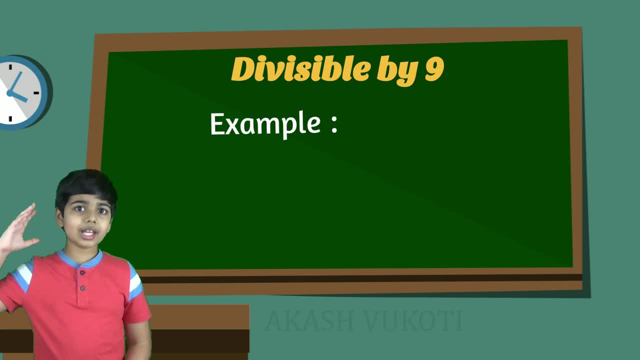 digits of the number, and if the result is divisible by 9, then the entire number is divisible by 9.. For example, let's take 1872.. 1 plus 8 plus 7 plus 2 is just 18, and 18 is divisible by 9.. It's 9. 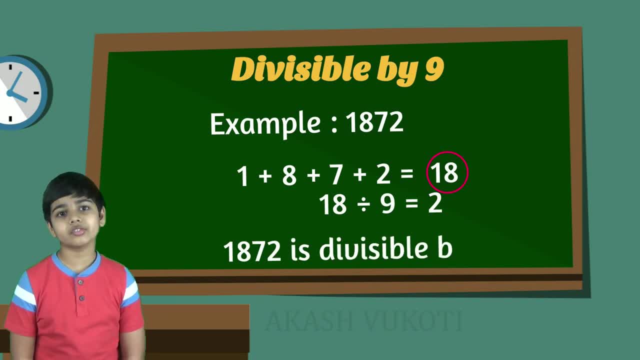 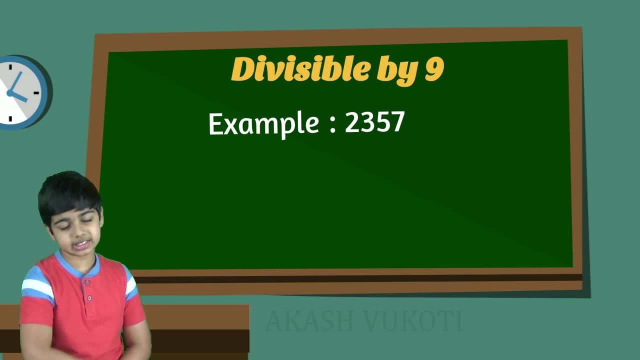 times 2.. So 1872 is divisible by 9.. However, let's try taking 2357 instead. Now, 2 plus 3 plus 5 plus 7 is 17, which is not divisible by 9.. So 1872 is divisible by 9.. Now, 2 plus 3 plus 5 plus 7 is 17. 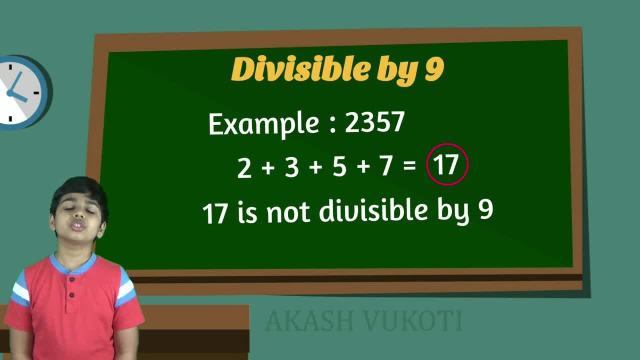 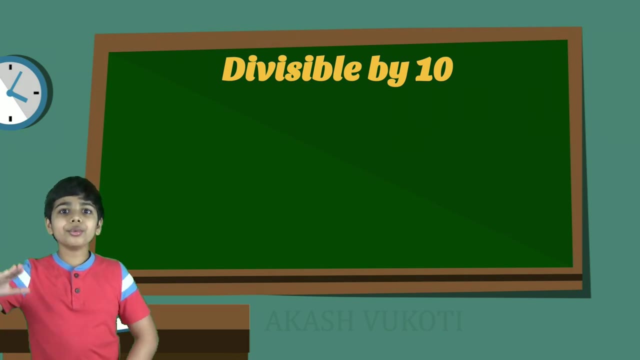 which is not divisible by 9.. So 1872 is divisible by 9.. So the original number 2357 is not divisible by 9.. And finally, let's take 10.. And this is one of the most easiest, because all you have to do: